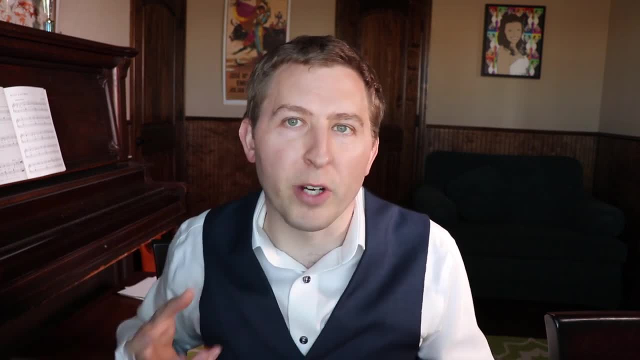 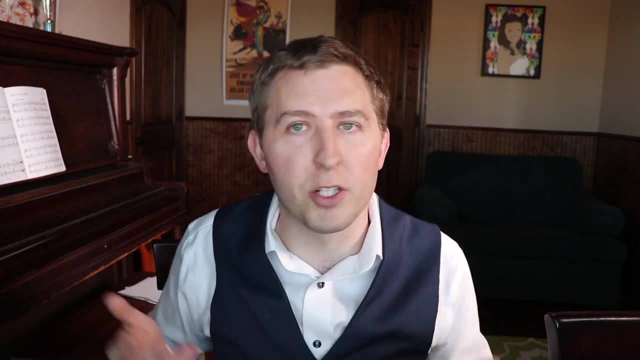 of how do you actually do this in practice, In theory, in trying to find a book that's theoretical enough and rigorous enough that you learn how to do Stochastic Calculus on its own, without applications to a specific problem, but also being applicable enough that you can quickly tie it to different fields. 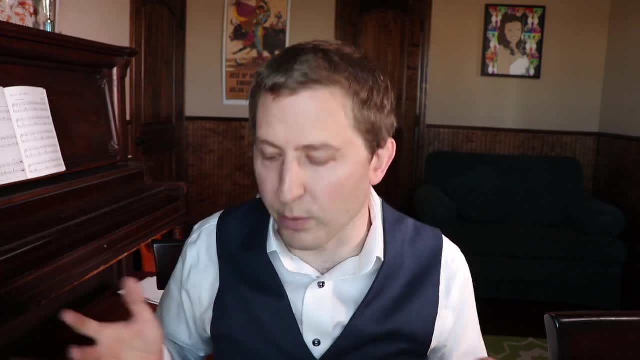 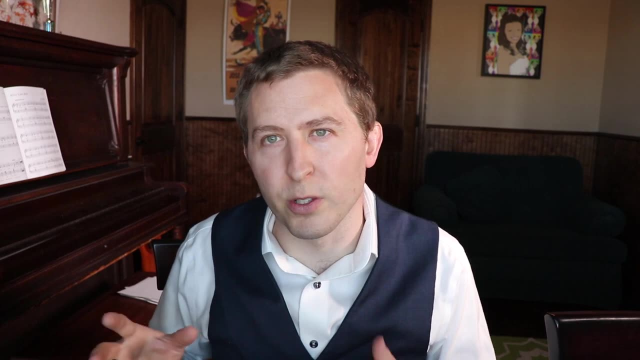 of study. this book kind of hit all those check marks for me, And in the back of the book it has finance applications, it has biology applications and it has a few physics examples- applications here as well. So I emailed Dr Clavana and I asked him for the book. 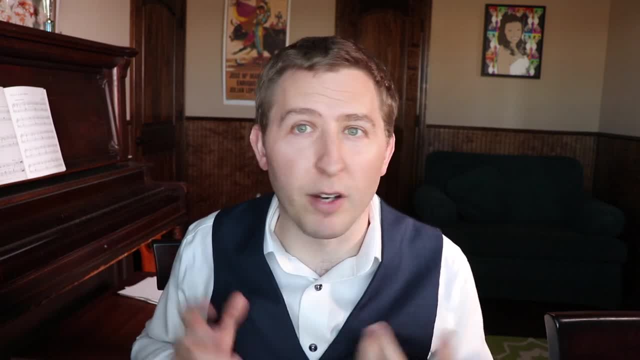 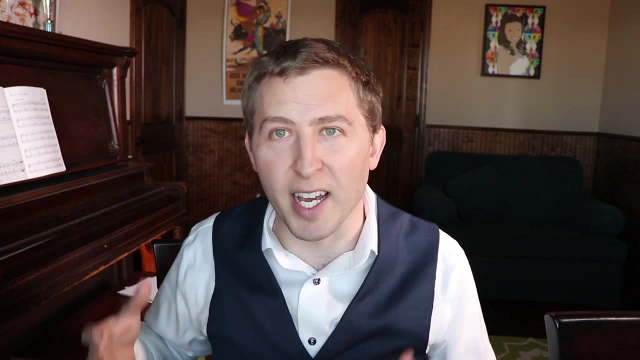 right And he said: you know, this is a book I really want to read it. I have a channel, I do book reviews And he was really happy to actually provide me this book So he mailed it. He teaches at Menash University in Australia, So the book was actually mailed to me from. 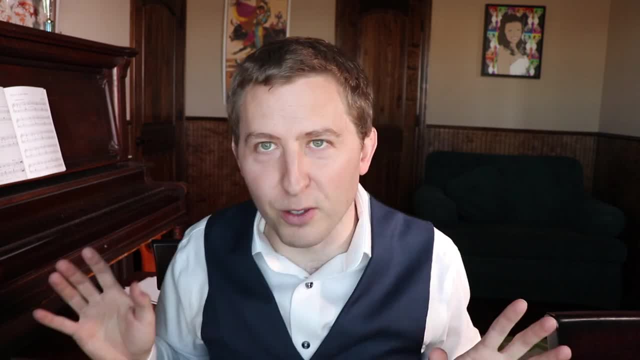 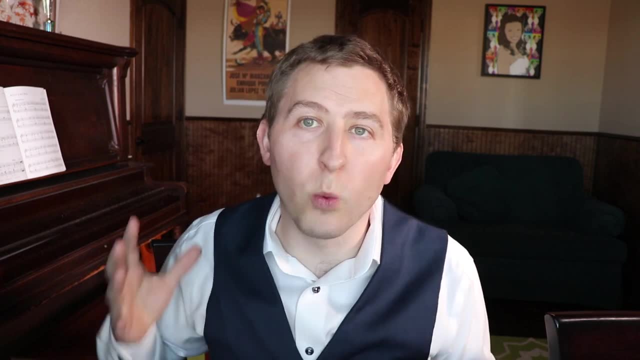 him in Australia to the United States. So, out of full disclosure here, this book was free, provided by the author, but I'm actually the one that messaged him wanting to review the book. Okay, so what do I really just love about this book? This is probably the best Stochastic. 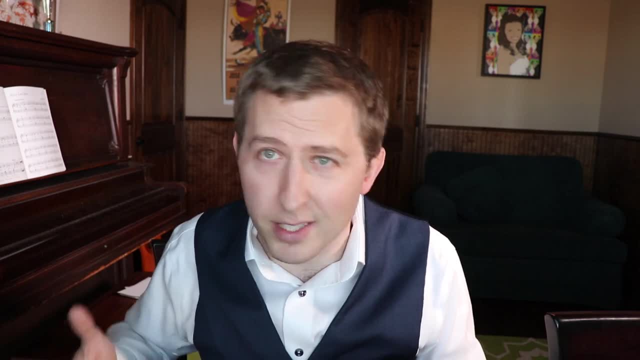 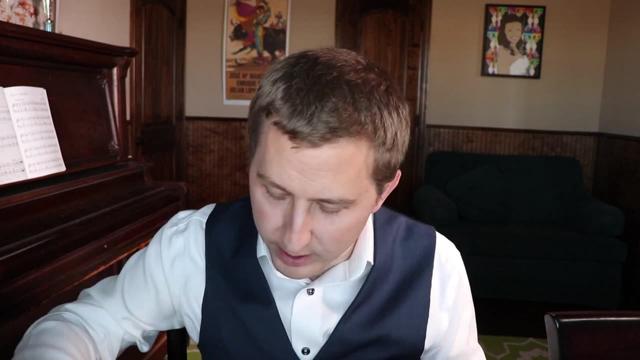 Calculus book- introductory book, right For Stochastic Calculus. This is the best Stochastic Calculus that I've read. One of the biggest things that I just really like is the layout of the book. So the book starts off with the preliminaries from calculus, then it goes into. 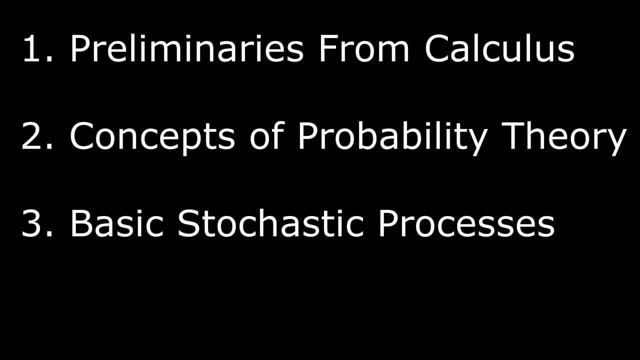 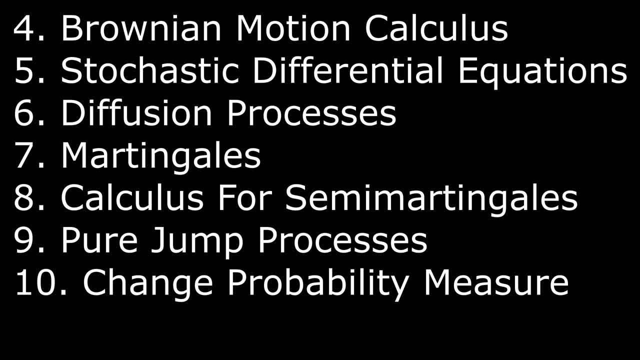 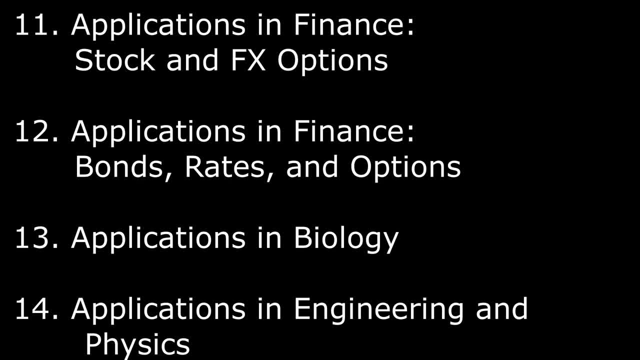 Now, the second thing that I love about Martin, I guess, is that he does really well. There are applications in finance, which has a few chapters in that: a chapter on biology and a really short chapter on engineering and physics. So I like the way that he builds. 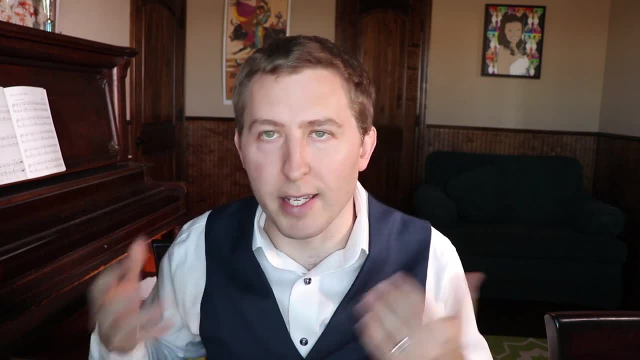 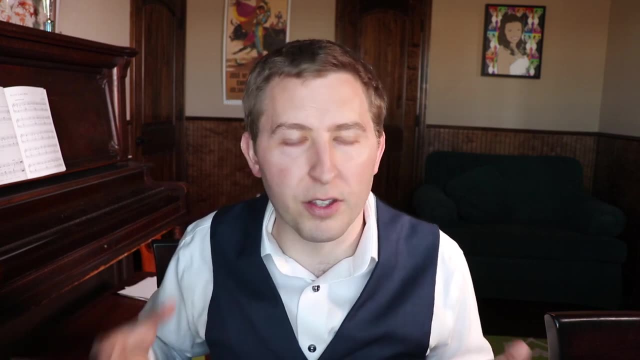 on the material and it kind of takes you from one topic to the next and a nice conceptual way that's easy to understand, like why we're going through the process we're going through With many textbooks. the authors don't think these things through. Given that he's a professor, 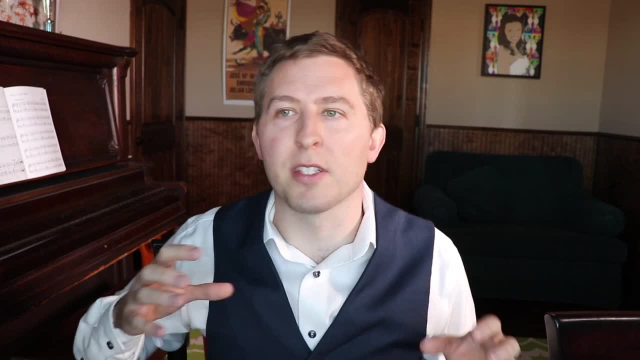 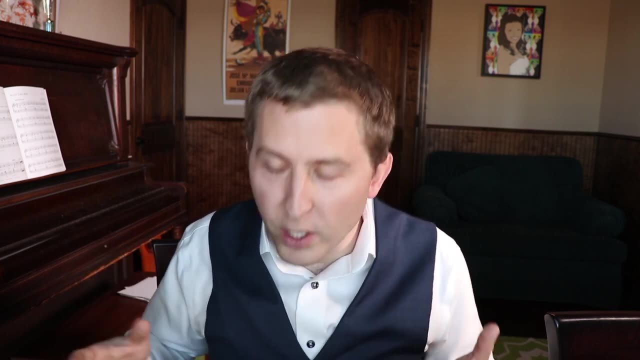 it seems like he's done a lot of teaching on this topic and he's actually layered this in a very kind of cohesive way way of putting it together. Now, that being said, I do not recommend this book for business majors. okay, You're going to need to take at least Calc 1 to Calc 3.. I would really really recommend you. 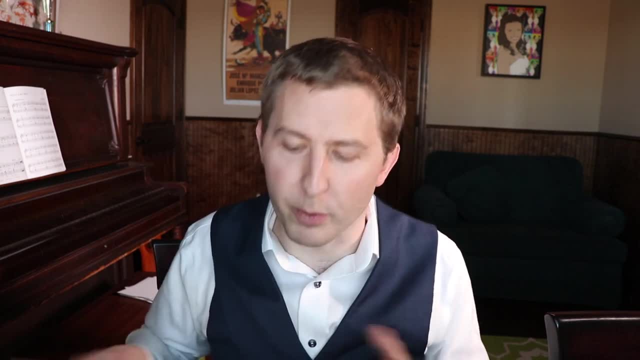 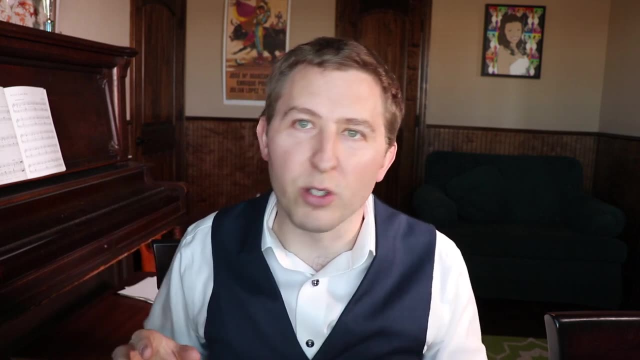 take Measure Theory as a course, or at least study Measure Theory or read some other book before you dive into this book. And then you need to take at least a few probability classes just to get going here. So I looked at reviews online. Some people are like: oh, this is not an introductory book. 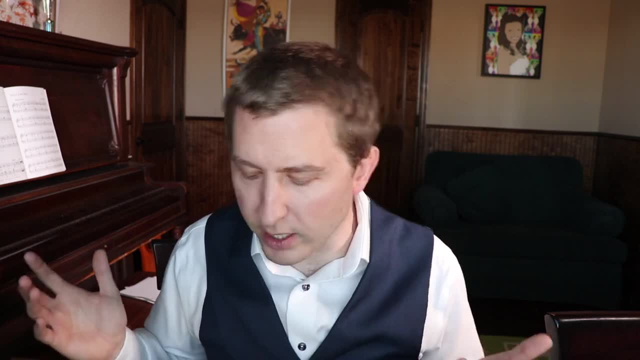 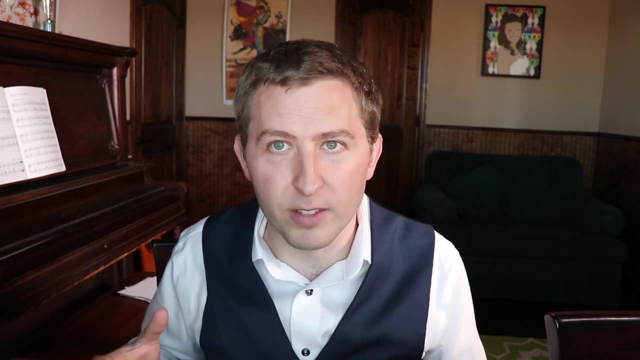 You know, someone even said they had a physics degree from a top-notch university in their country And this book was like unobtainable. It's hard to read. Stochastic calculus is a really challenging topic. okay, It's hard to learn, It's hard to understand- Even myself, right? 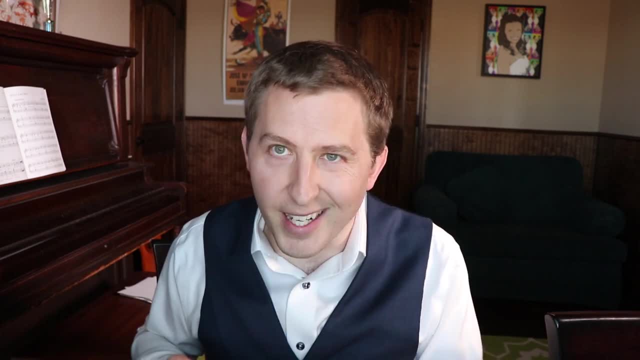 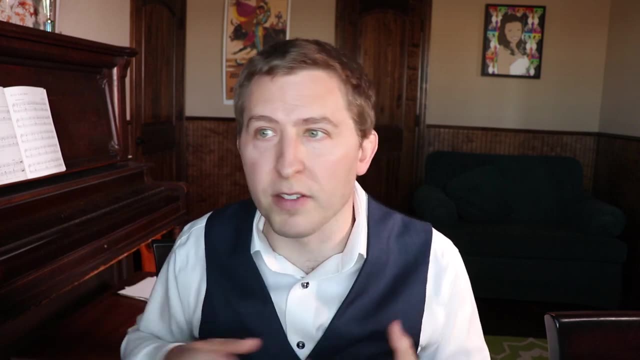 it's hard to grasp those ideas. But one thing that really excited me with this book is like reading through the book the presentation He does, mathematical kind of like derivations of some of these like lemmas and proofs, and how you get to things theoretically. These aren't easy. 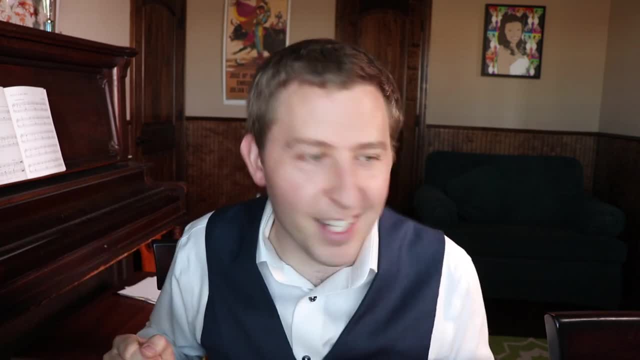 things just to learn. You don't just read the book and go, oh, I completely understand stochastic calculus. You don't just read the book and go, oh, I completely understand stochastic calculus And, like you know, I'm out the door building out exotic derivative pricing options. I don't know. 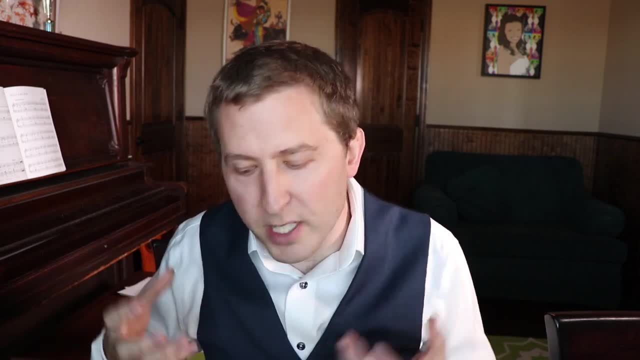 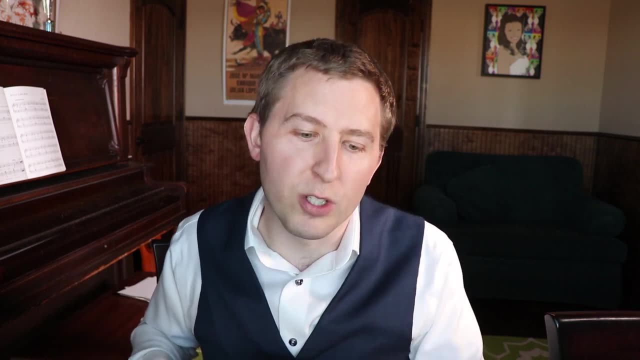 something like that. The book itself, though, it makes me think. It makes me really want to dive in deeper, And he references some papers and he has some exercises in the back, which I'm going to point out here too, something I loved about the book: At the back, there's select solutions. 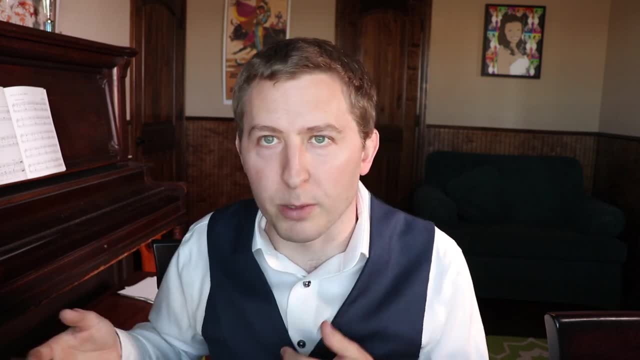 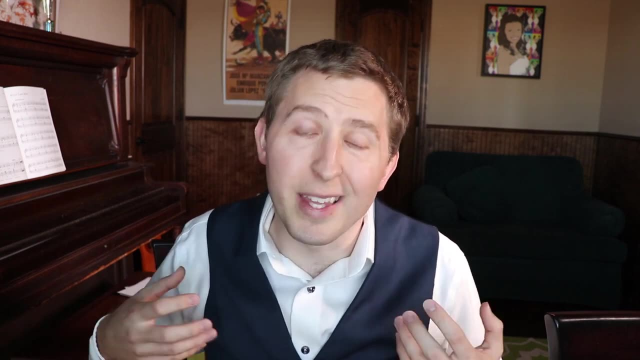 to some of the homework problems. So at the end of each chapter there are homework problems or exercises, And then he provides in the back solutions for those. So I like the way the book is set up. I think it's an amazing book. I think it's a great book. I think it's a great book. 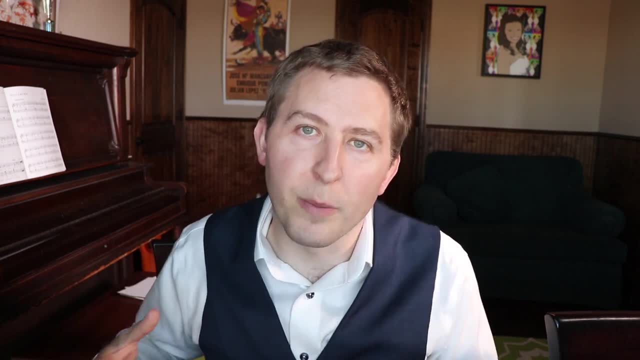 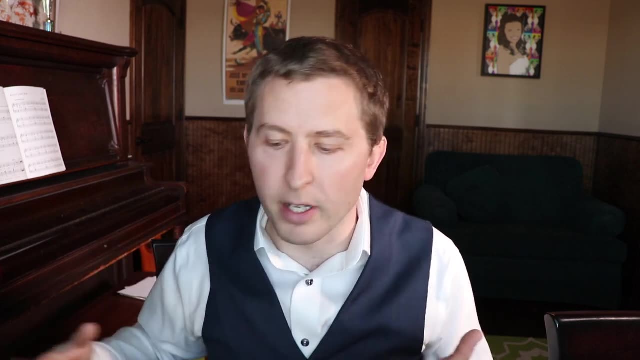 If it was to be used in a university for teaching, it's also something you could use for self-learning, because you can kind of wrestle and grasp the ideas. And if you need more background, you need more information. right, There are papers and academic sources you can. 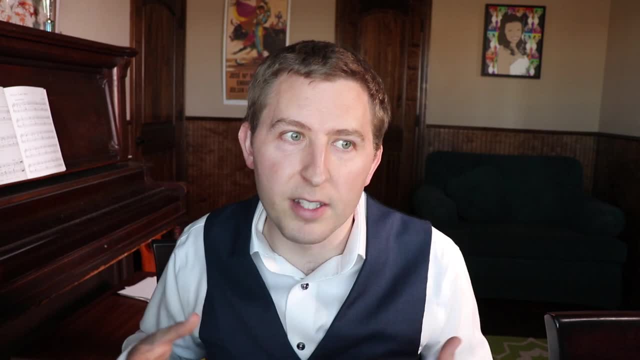 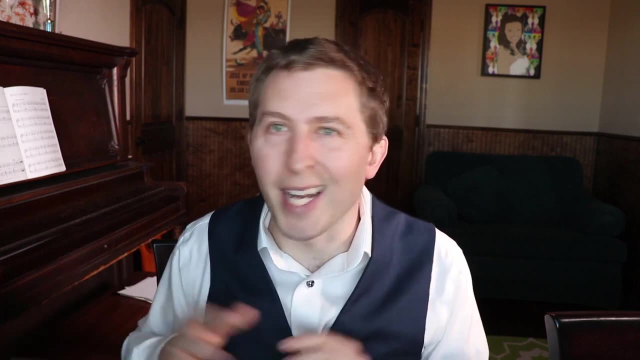 search through in this book And then you can also do the exercises and then check the solutions at the back right, Those select solutions. It's not all the solutions, but you can go and look at them and say, oh okay, like I didn't get the right solution and kind of work back and work through. 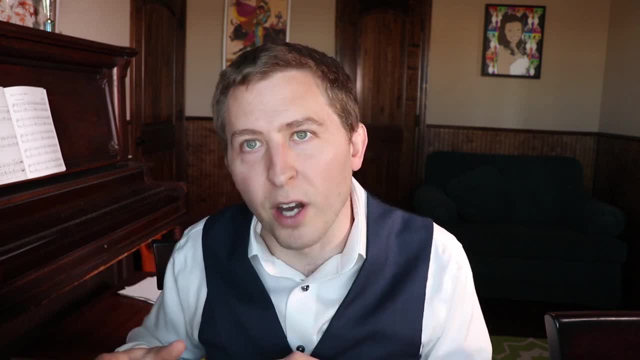 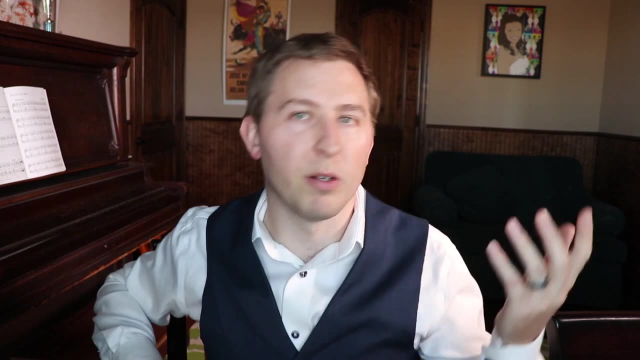 it. This book is for someone who wants to be a real quant. This is not a book that you're just going to pick up and like, read overnight and understand stochastic calculus And then I don't know it's one and done. But the things I liked about the: 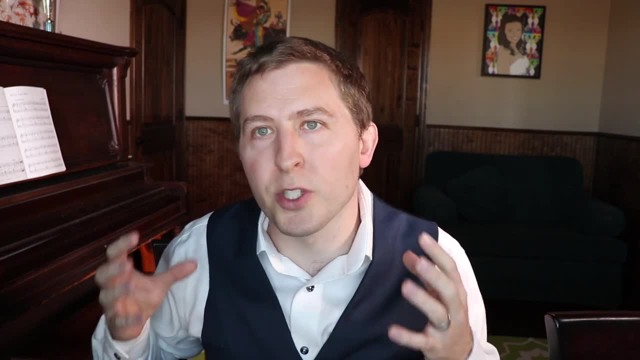 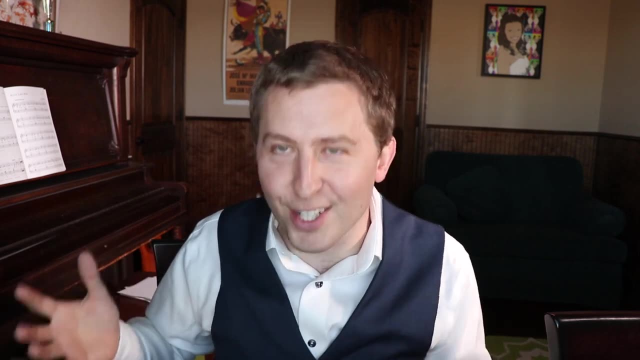 books I mentioned. the layout of the book is amazing. The examples, the proofs, the rigor, the mathematics in the book are amazing. Again, it's not going to be the most advanced book, right, It's called Introduction to Stochastic Calculus. But, that being said, it does assume. 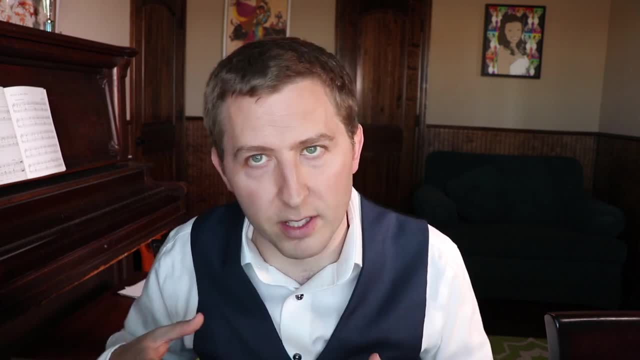 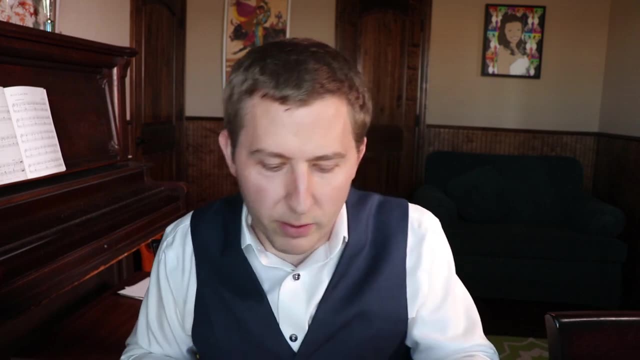 you have a strong background in math and probability before you dive into this right. Those are those two components. you need to really learn stochastic Calculus. And then there are some. there are two chapters in the back here which I'll mention. 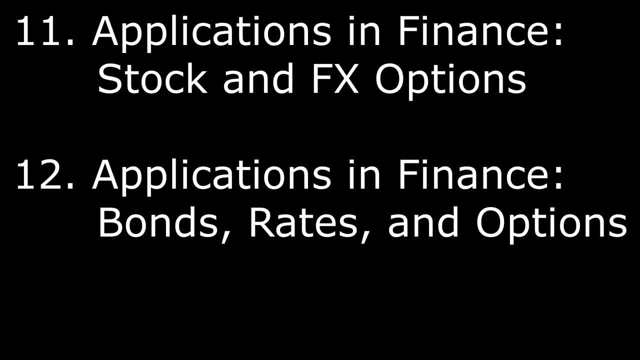 And they are Applications in Finance, which covers stocks and FX, so foreign exchange options, And then the other chapter is Applications in Finance: Bonds, Rates and Options. He covers a lot of just the really basic bare models you're going to use for stochastic calculus here. 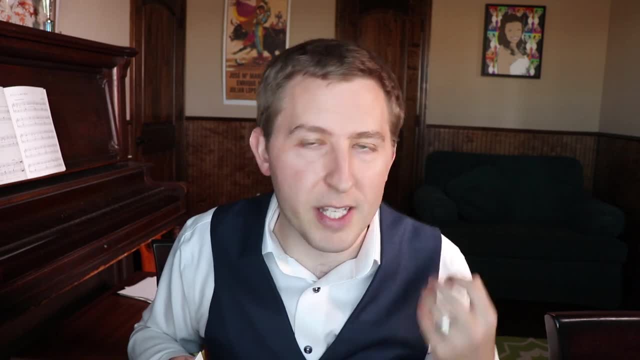 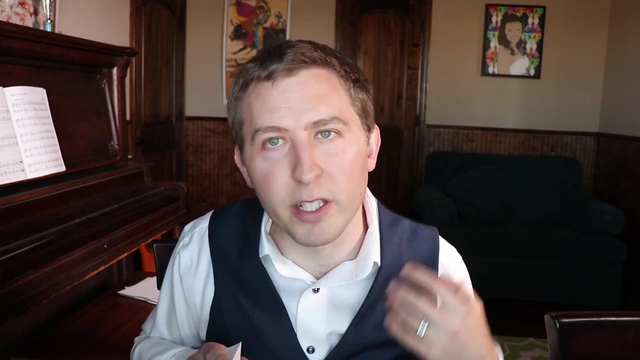 He does a great job of kind of breaking them down. Again, the focus of the book is not finance, it's learning stochastic calculus. But I think once you do the first 10 chapters in here and you really grasp the material, applying it to finance is not going. 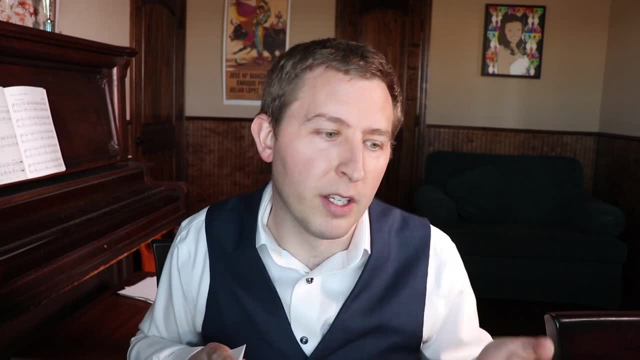 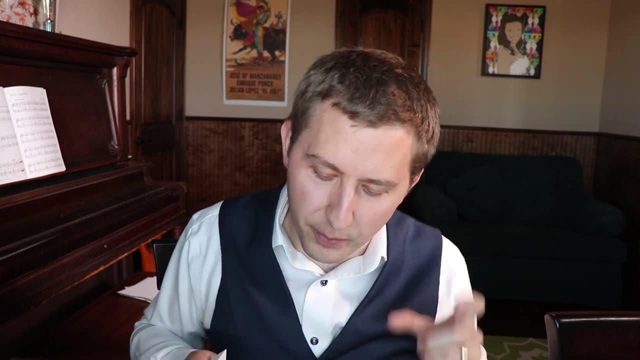 to be as challenging as coming from a- you know, uneducated perspective of stochastic calculus and then trying just to learn it and apply it to finance all at once. There's a big section on biology and a really small section on engineering and physics, But my favorite section of this whole- book is actually the biology examples. The reason for this is biology is a hard science And so, yes, there's uncertainty within different things. Again, my favorite part of this book is actually the birth and death process, which is section 13.3.. 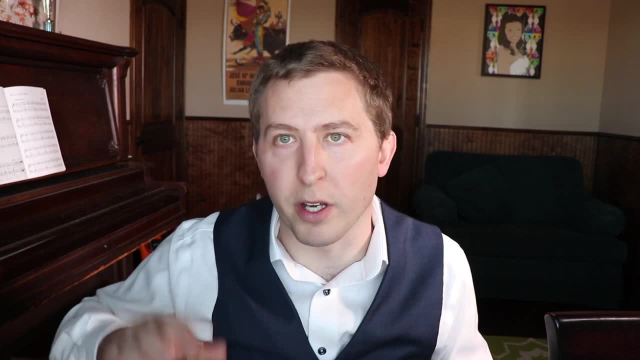 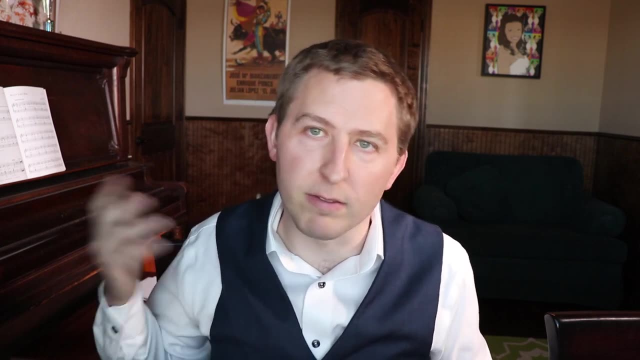 And also going into the next section, which is actually on modeling cancer and mutations. For me, biology just makes more sense. So I have a finance degree, an undergrad. I come from finance, I get it, I know I've taken the classes in financial engineering programs, But I just 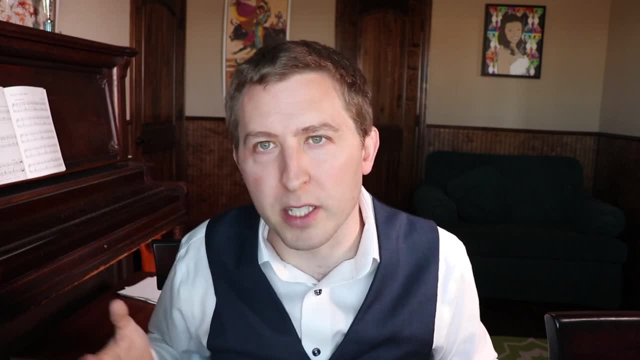 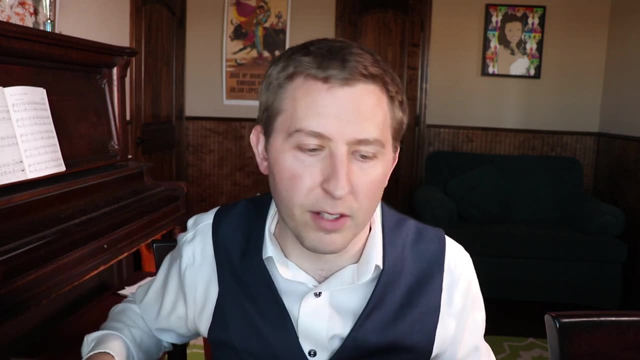 think that applying this to a scientific biology perspective made it a little more clear for me And it helps to kind of see how you apply this outside of science And I think that's really important. So one of the big detriments, I think, for a lot of programs. so not for this book, but 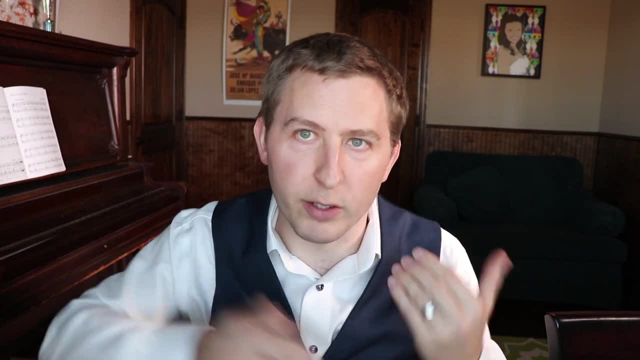 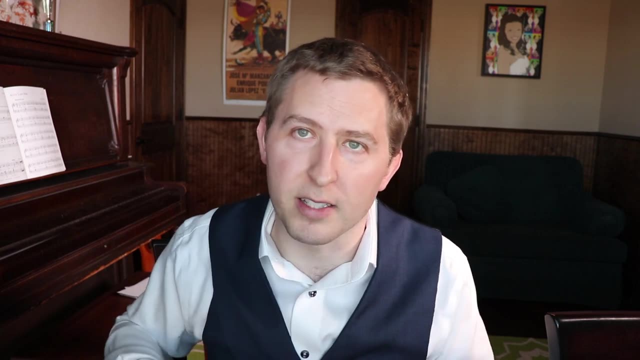 for a lot of programs is that students only learn the rigor of like, repeating and memorizing equations within an application. So specifically finance This book, though I think does an amazing job of stochastic calculus. I love the thoroughness of it. I love the segues, as I mentioned, like 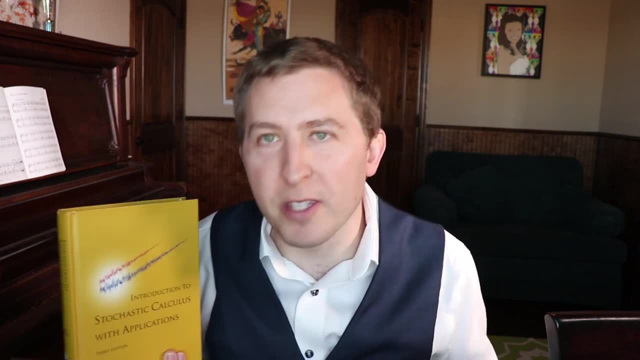 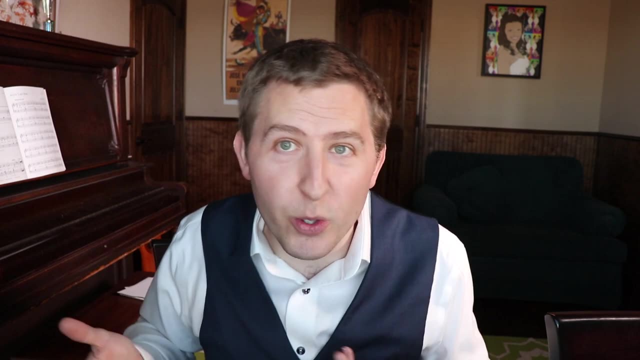 I can't say enough good things about this book. I'm up in the air on exactly how to rate this out of five stars. My first initial reaction was it has to be a five star book because I've I've enjoyed reading it so much. It's one of those times where I sit down here at my desk. 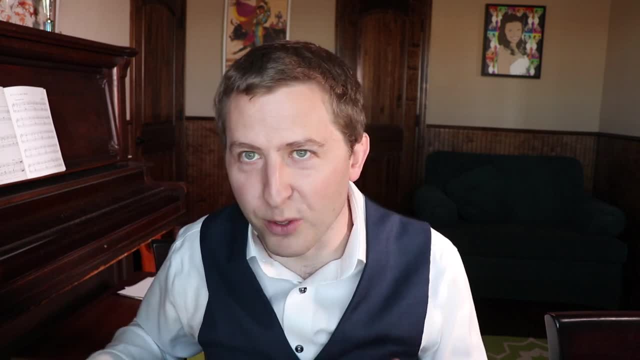 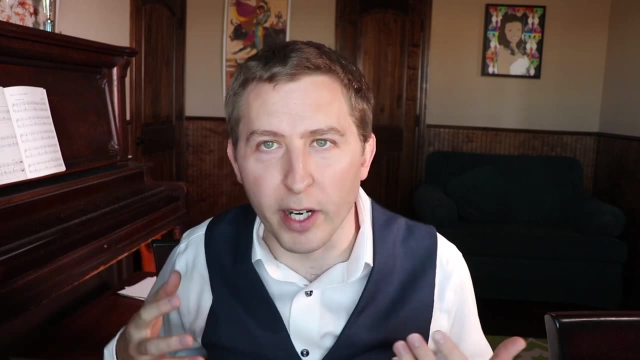 you know, cameras off and everything, And I'm actually like reading through the book And I have a sheet of paper and a pencil next to me and a big eraser And I'm like working through some of it and trying to grasp the ideas better, trying to really see where it's. 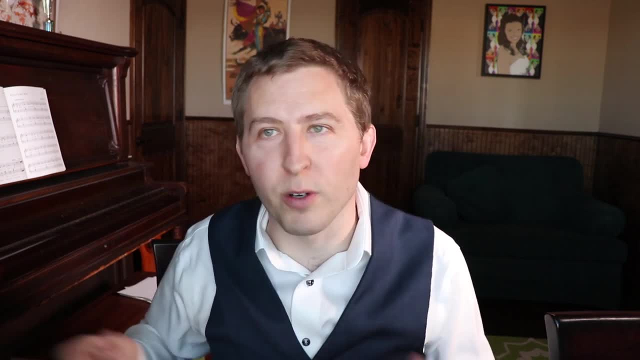 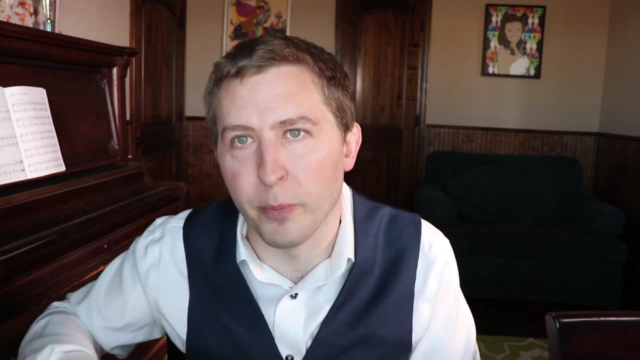 coming from theoretically and thinking about it deeper And again, of course I'm using, you know, the internet and searching things as well and adding into my studies. But it lays a great foundation of how I could study with the book. It's enjoyable. I have not covered every aspect. 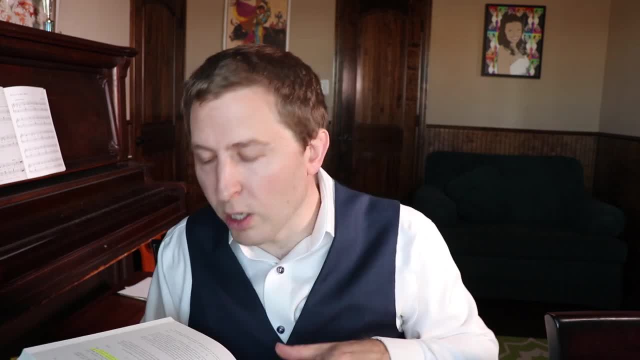 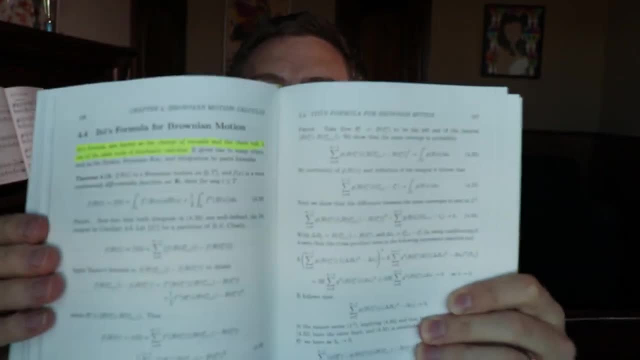 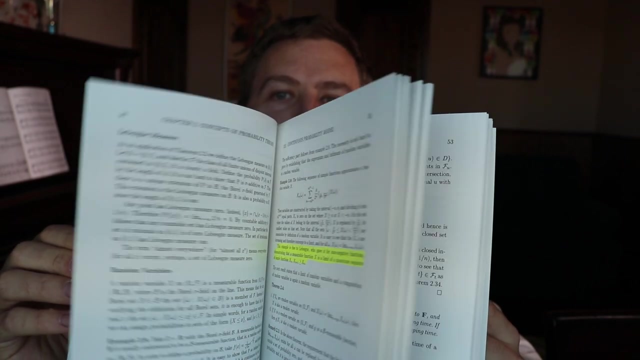 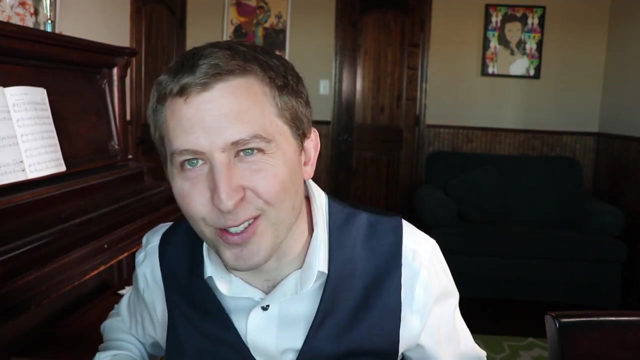 every page of the book itself. I'll show you guys here, I guess, briefly, if I can flip through this. So, as you guys know, yes, I I actually read the books and I highlight in them and I take notes in them. Again, I I just thought it's just a well put together book, So I can't say anything. 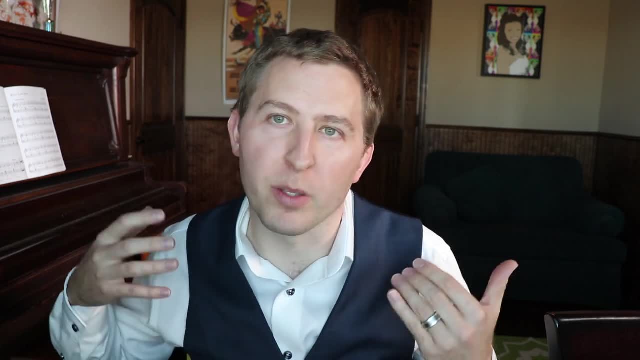 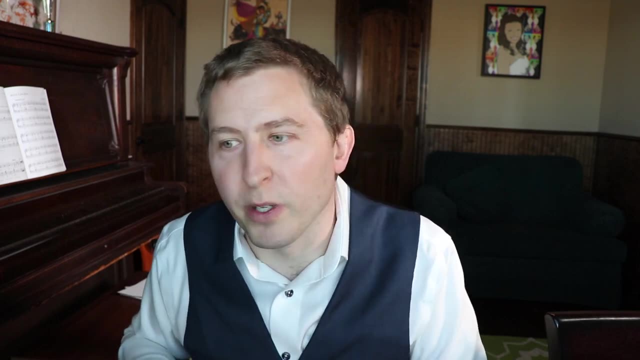 else great about besides that. I did like one thing: it laid out kind of the principles and assumptions behind classic processes. I don't see this a lot in other books. Again, I just absolutely love this book And then I thought you know. so on the rating side here five star has to be five star And I 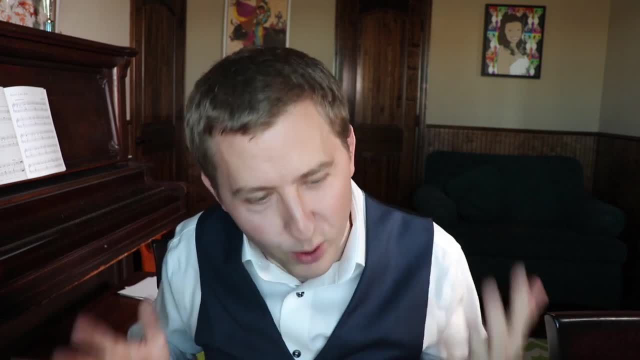 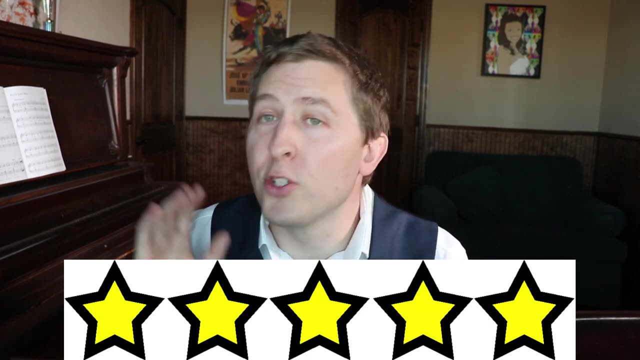 thought: but is it perfect? right? If it's not perfect, maybe I should give it a 4.5, telling you half star increments. But I think, overall, guys, I'm going to give this a five star for the book. Again, I do not recommend the book. please don't buy the book If. 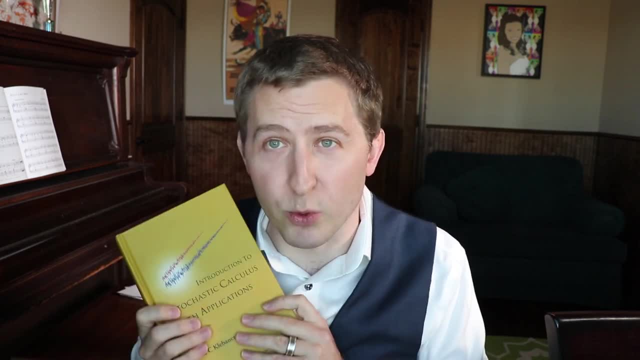 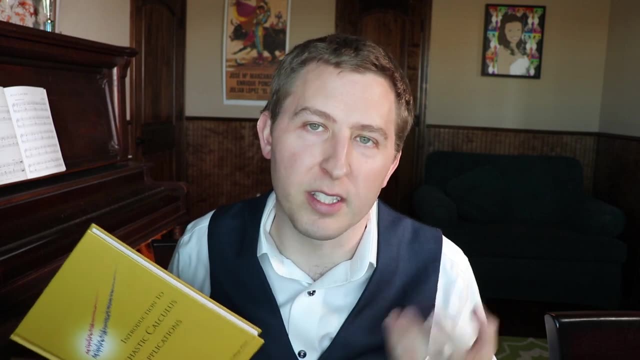 you're from a business background, you're going to spend money on this and it's going to be really, really challenging. You know, I guess, fully grasp- at least at that point, at an expensive mistake- what stochastic calculus is and the complexity behind it.